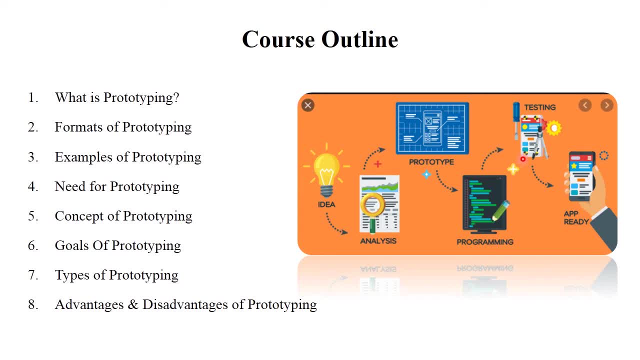 ideas, then prototype, then programming, testing and at last, your app will be ready. So this is just concept regarding prototyping techniques. So let's see. the first point is what is meant by prototyping. Next, So what is prototyping? So what is prototyping? Prototyping is a. 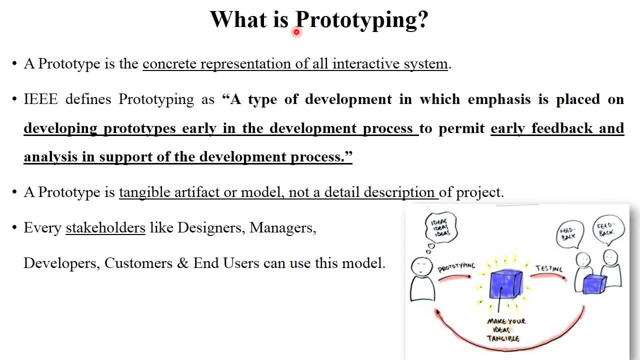 form of prototyping. We all are familiar with the word that is prototype. Prototype means one kind of structure or model, right. So prototype is concrete representation of all interactive system. IEEE defines that prototyping as a type of development in which emphasis 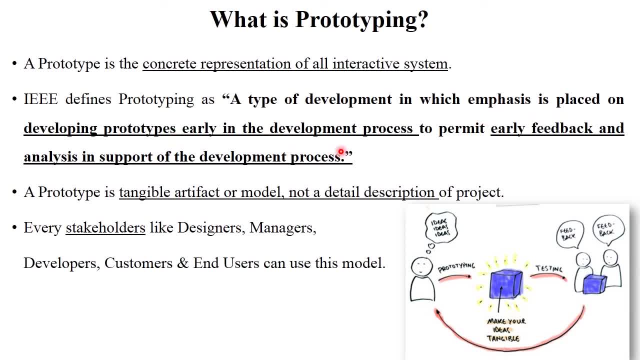 is placed on developing a prototype early in the development process. You should make a prototype of the particular model before the development process Next. So what is prototyping? So what you are doing now is we are talking about prototype. So in this, 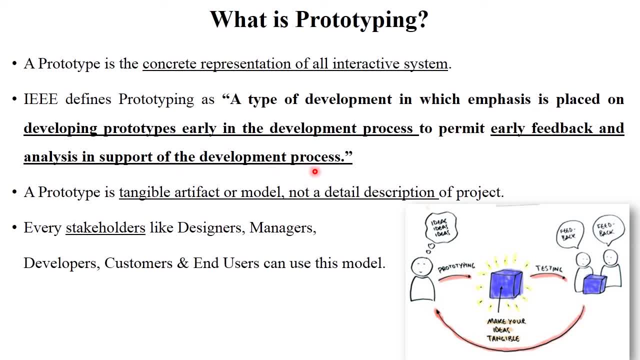 on the development process. we are in the process of developing a prototype, So you should be trying to understand what is prototyping Okay, And to permit early feedback and analysis in support of the development process. So, by using or by helping prototype, you should. 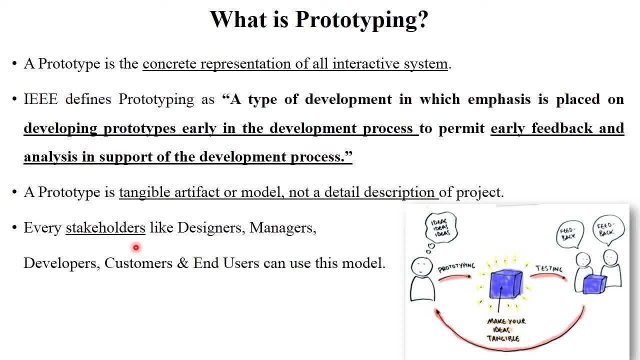 analysis what exactly your system will look like in future. So prototype is tangible. end user can use this model. so prototype means generally structure and model how your system would be look like in future. this concept is called as prototype. see here the customer or the particular designer or developer. they have so many ideas regarding that, so make one prototype. 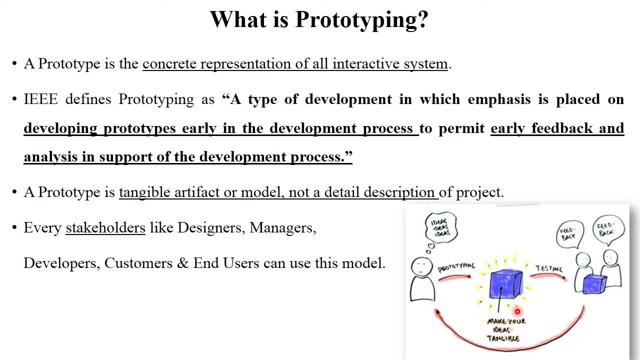 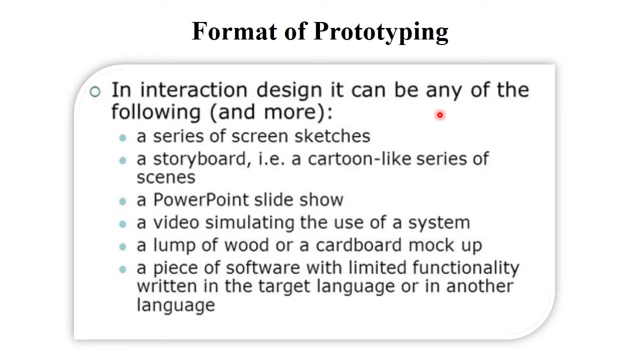 make your ideas tangible. this means that make the particular prototype of model. after that there is implementation of that particular model and testing process will be done right. so this is the concept of prototyping. next, formats of prototyping in interaction design. it can be any of the following format: you should make a particular screen or sketches of the 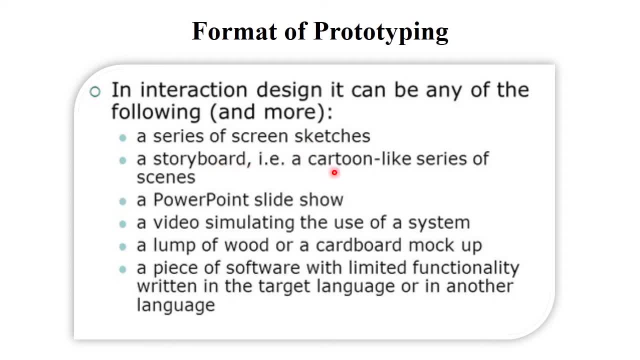 particular model. right then, storyboard. storyboard means animation, videos or how your system will be look like in future. okay, for example, sign up screen. after sign up, there is login process and after the next, the particular screen will be open. so this kind of scenarios: okay, this called as storyboard. 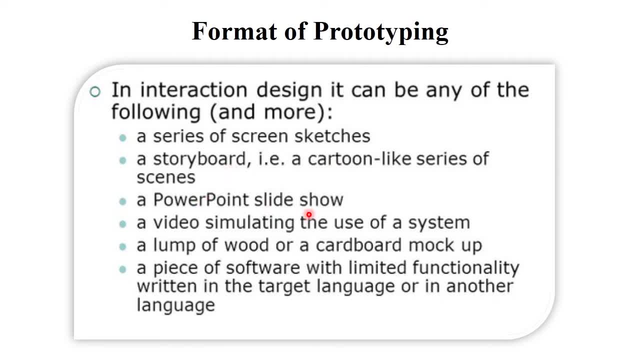 then powerpoint slideshow: you should make a powerpoint presentation of your system, okay, before implementation, how your system will be look like. then video simulating use of the system. lump of wood or cardboard mock-up- these things generally used in architectural field. right architectures used or make a particular prototype or model before the development process, right? 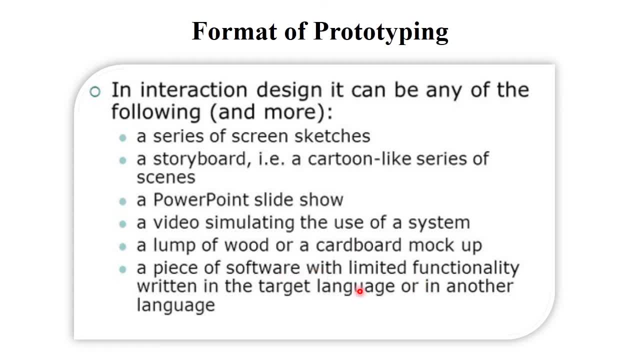 then piece of software with limited functionality, written in target language or in another language. you should make a just one kind of algorithm or structure how each and every screens, designs, models are work okay. so this kind of formats are used for the prototyping, or should make a prototype of the. 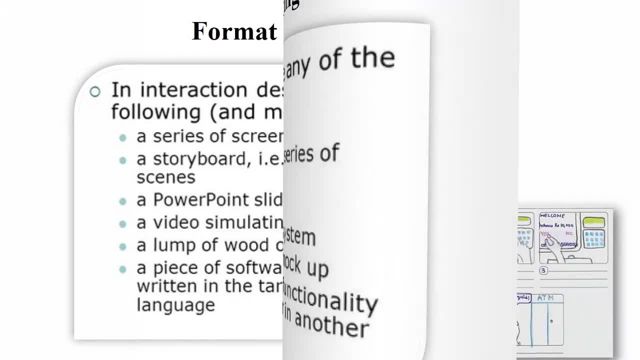 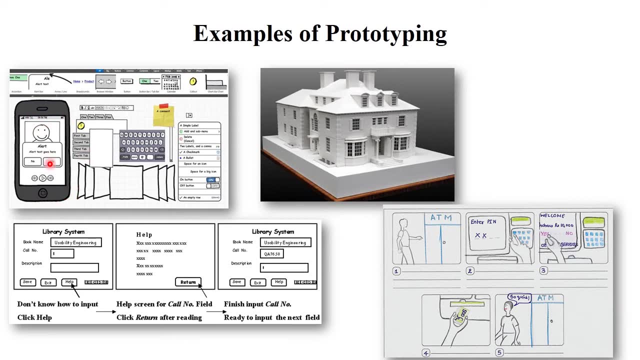 particular model. right, okay, of mayo. that's for next left is that again get the right asked that soon sends before to the village Like library system project. So first book name their description: Again there are some options are available, help, And after click on help button it goes to next screen. Right, Again, it goes to next screen. So this kind of structure. It's easy to analysis How your system would be look like And it's easy to understand each and every stack holder in your development process, Right. 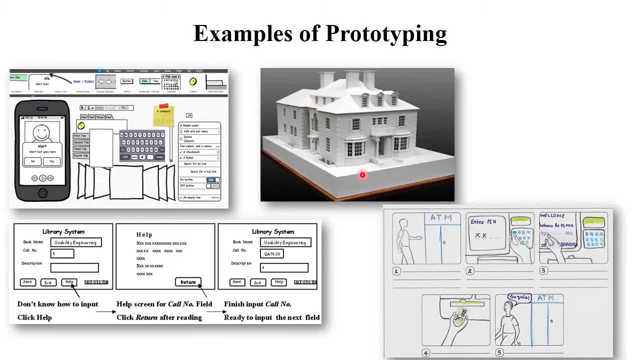 Again, this is another example of prototyping. This concept generally used in architectural field. Okay, Before they make a particular model of that particular home, or the hospitals, colleges, etc. Or the particular building Right Now, this is again scenario of ATM machine. How exactly ATM machine will be work. This again another prototype, according the numbering format. Okay, So these are the some examples of prototyping. 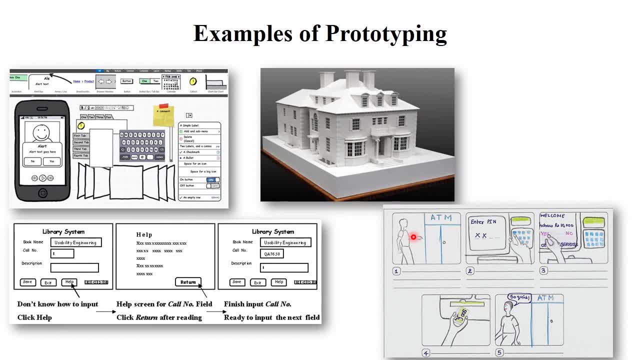 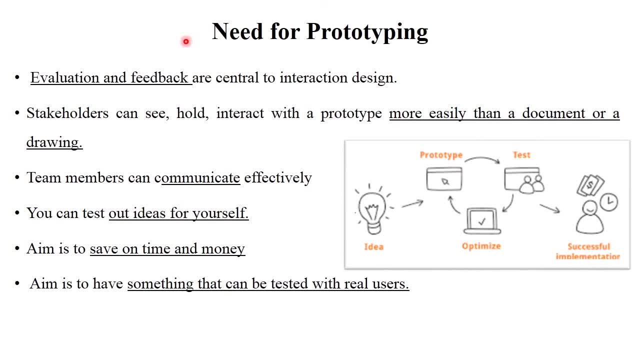 So prototyping is one of the most important step in development process. Clear Next Need of prototyping technique. So the most important thing is: evaluation and feedback are central to interaction design. Okay, So through prototyping you get feedback And you should make again changes in that particular model, Right? 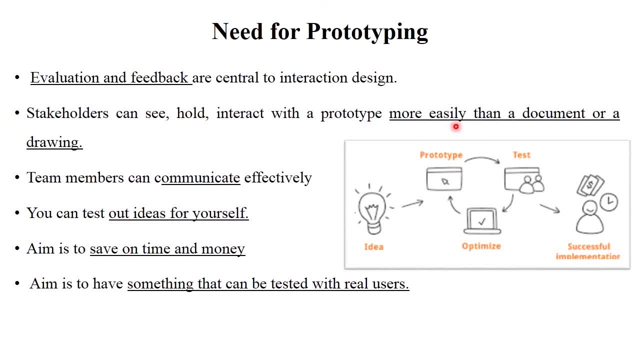 Then stack holders can see hold interact with prototype more easily than document or drawing. So prototyping is most easiest way as compare to documents or the drawing Right. Team members can communicate effectively Through prototype. you should generate a new idea Again. you should implement those prototype Right. 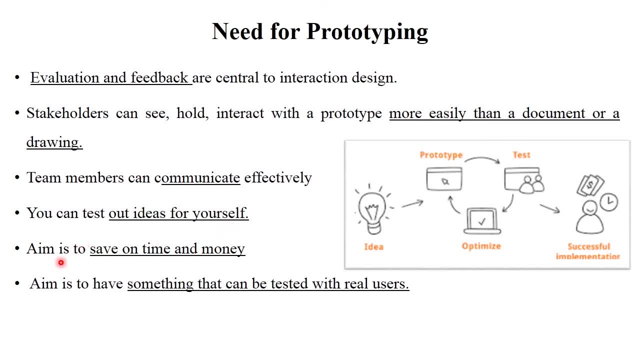 You can test out ideas for yourself. So the main aim of prototyping is save on time and money. Again, aim is to have something that can be tested with the real users. So suppose you should make a prototype Before starting up the process ahead of time. So prototyping is the most important step in development process. Okay, Next. 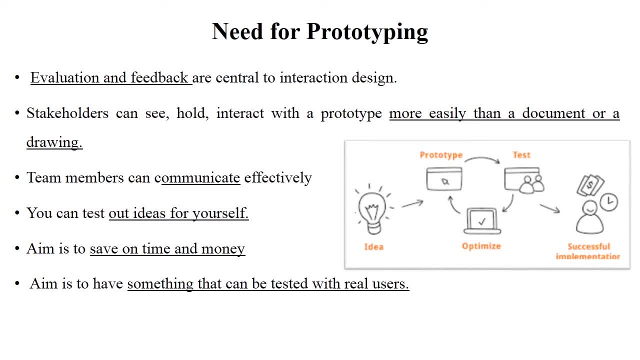 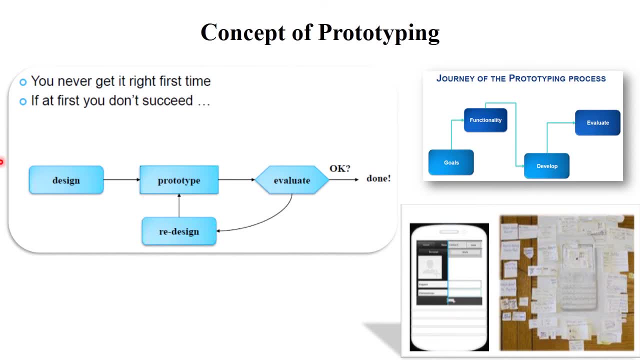 So prototyping is the most important step in development process. Again, you should make again changes in that particular model, Right starting the development process. So it's easy to understand, Right. Next, Next, concept of prototyping: See here this diagram show the concept of prototyping techniques. The first: 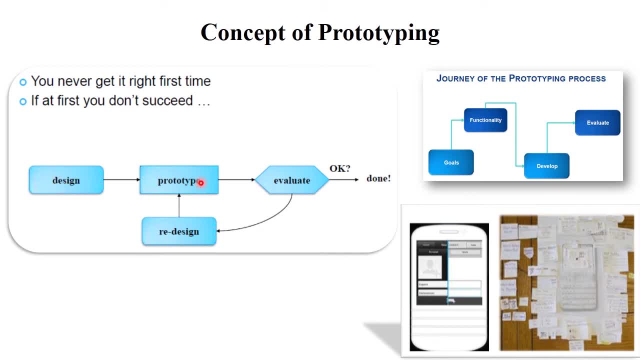 phase is design phase. Right After that there will be prototype according the design requirement. Okay, And after that evaluation or implementation- Suppose there are again some changes are needed in this implementation phase, Again it redesign the prototype Again, make, evaluate it Again. 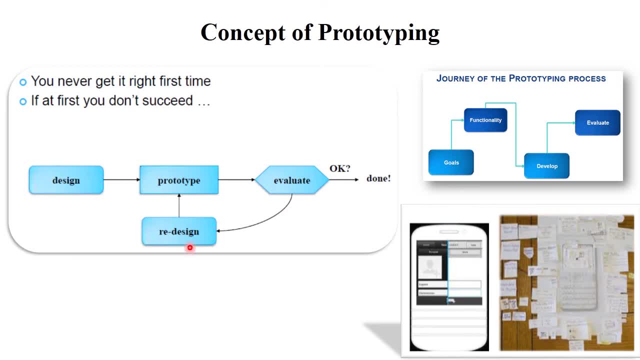 redesign it Again, evaluate it. So prototyping is a loop sector or loop features are available here. Okay, So, as per the requirement, as per the implementation, you should make a particular prototype or design of that particular product, So your customers or users will. 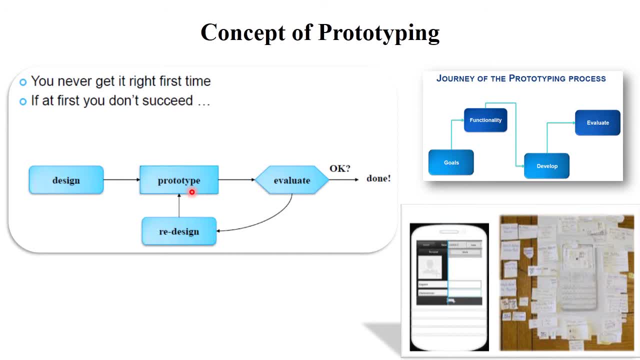 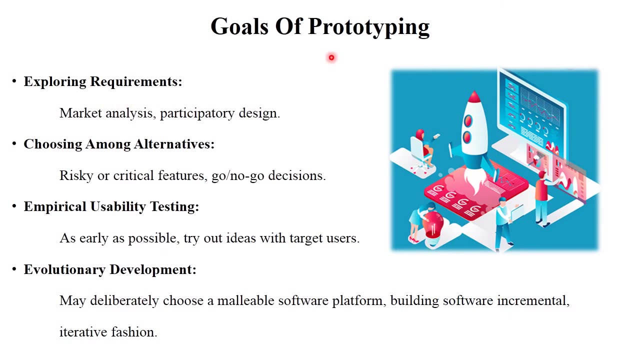 get more satisfied about your product. So this is the journey of prototyping. Now the goals of prototyping process. The goals, functionalities, development and evaluation- These all things are included in prototyping techniques- Clear. Next, Now the goals of prototyping techniques, Why we use prototype. So first main goal: 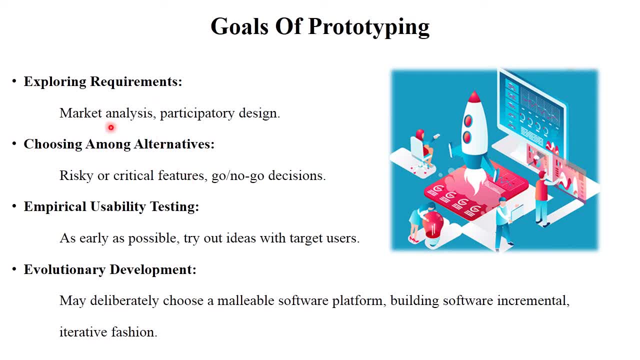 is exploring requirements. As per the market analysis, as per the recent trends, you should make a particular software or particular model. This is one of the most important feature of prototyping. Next, This is the goal of prototyping techniques- Then choosing among alternatives. If you make. 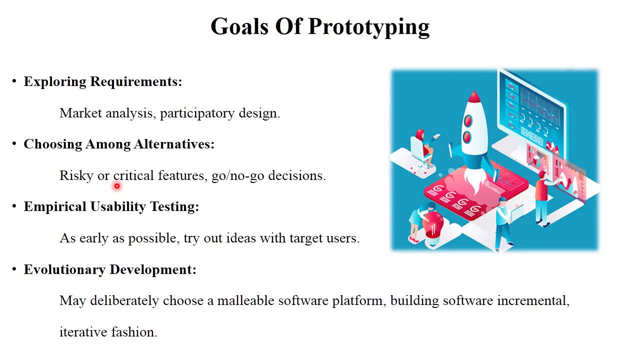 a particular prototype so it's easy to identify what will be the risk factors in that particular model. So you should decide and in prototyping phase only the particular decision is wrong or right, or particular features are will be added in that particular model. That will. 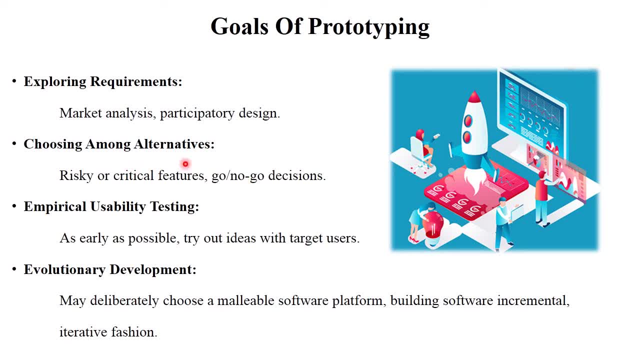 be wrong or right, Right. So this is the choosing among alternatives. The next, empirical usability. Empirical usability testing. So as early as possible, try out ideas with target users. You should arrange or implement different types of ideas on prototyping model Evaluationary development. 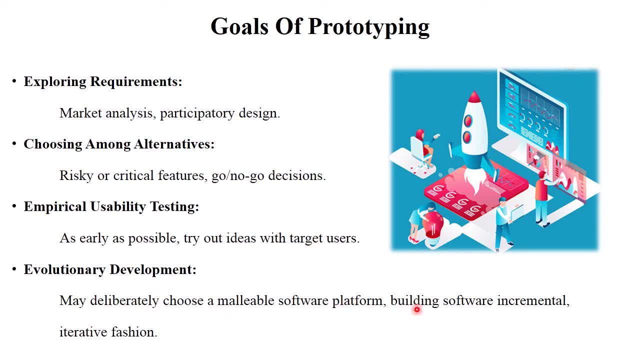 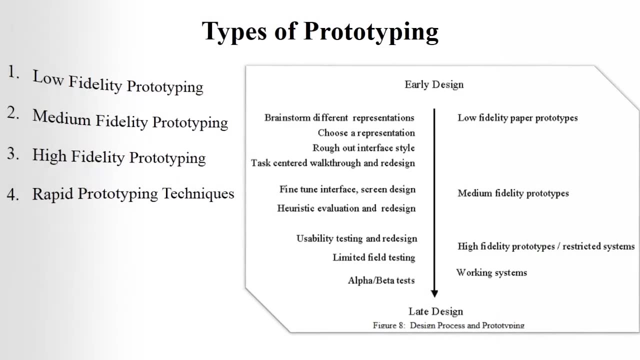 May deliberately choose a malleable software platform, Building a software in incremental and iterative fashion. So through prototype you should make easy for developer or the programmer To make a particular software or product Right. Next, Next type of prototyping. So prototyping is generally a brainstorming process. 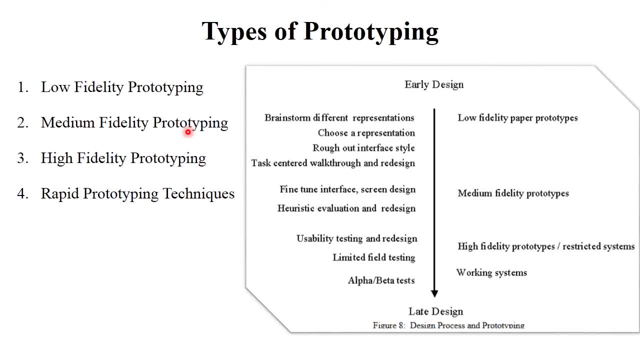 You should arrange a new ideas on that. Mainly, there are 4 types of prototyping technique, That is, low fidelity prototype, Medium fidelity, High fidelity And rapid prototyping techniques. In the next video I will explain in detail all the types of prototyping techniques. That is part 2. 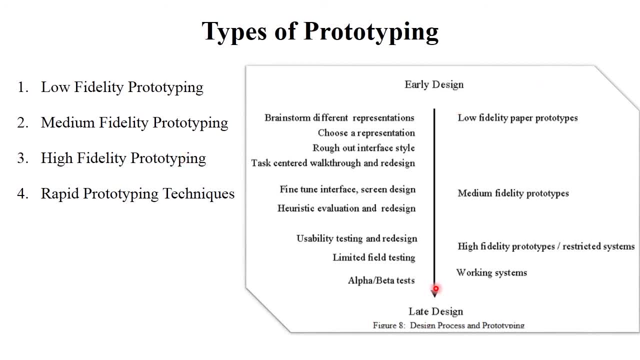 Okay Now this is just structure of the types of prototyping And this is the content of the screen design. I will give you just overview here. That is: low fidelity prototyping means Use paper or pencil for rough interaction styles. Medium fidelity prototyping means To develop a particular screen design here. 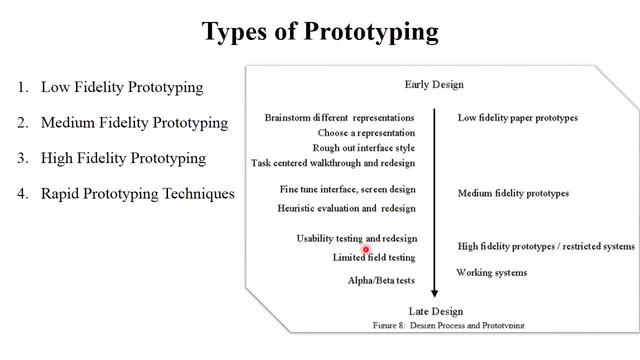 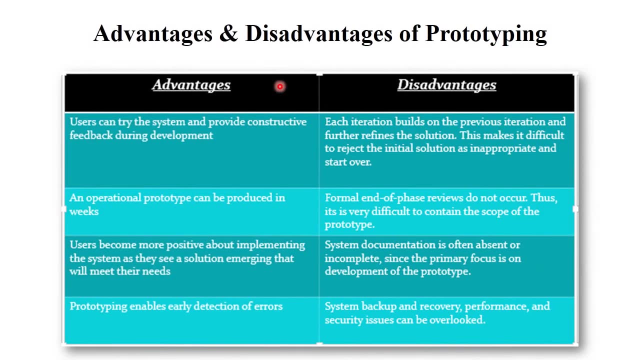 Then high fidelity means actual implementation, Usability testing, Then alpha beta testing. All things are generated or implemented in high fidelity prototype. So I will explain with examples in detail in the next video. next advantages and disadvantages of prototyping. so there are so many advantages and again disadvantages of that. so according the 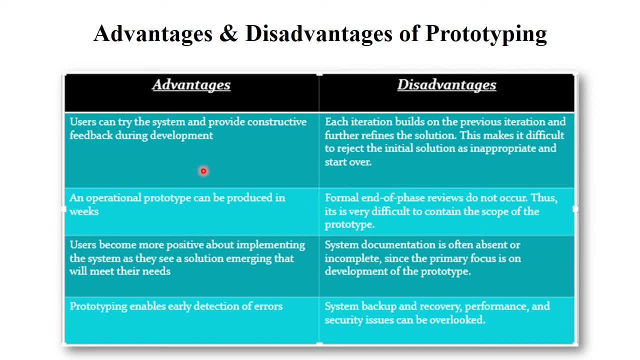 requirements in companies or in the industries, they should use a prototyping technique. so the advantages of prototyping is user can try the system and provide constructive feedback during the development process because real users are involved each and every phase of software development life cycle. then operational prototype can be produced in week. you should make a prototype more.